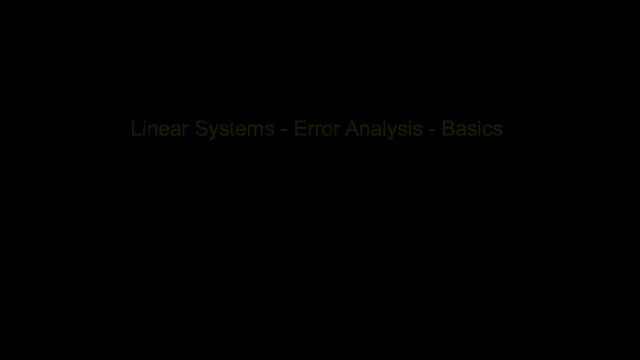 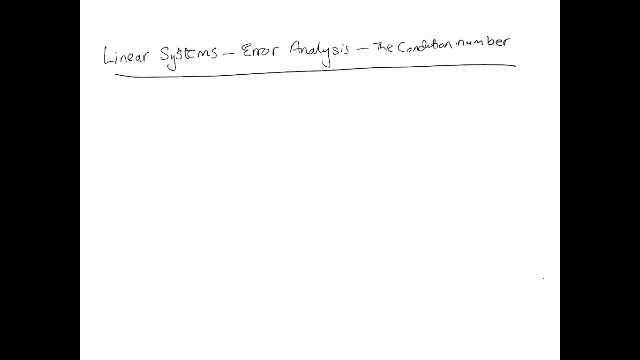 So in this video we're going to look at the concept of the condition number, because we are looking at linear systems. we've been having looking at them and now we need to start looking at how do we actually compute the error? how, how good is our solution, even in the direct methods, as you would? 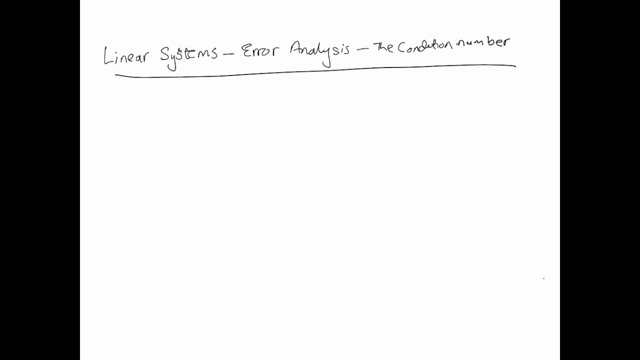 have seen in scaled partial pivoting or partial pivoting. why is there a need to have these is because we clearly see that there is. even in direct methods, our solutions are still approximate. they're not, in fact, exact, so this means not in the absence of the exact solution, how do we actually 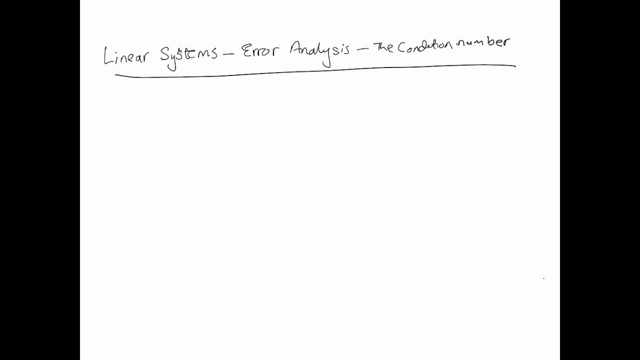 get an idea about how good or bad is our solution to answer this, we. this is where the concept of the condition number comes in. now, in order to get to the condition number, let's define certain things for the sake of getting to that definition eventually. first of all, we'll call x hat the. 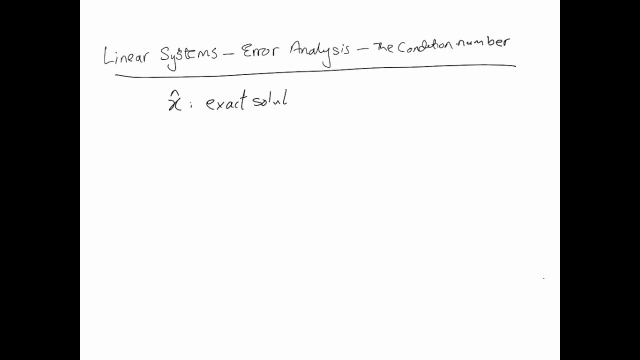 exact solution. okay, for the purpose of this video. so x hat is, in fact, we call that the exact solution. so, of course, an underline under it, meaning that it is a, it's a vector, so this is a vector. now, remember, our target is we are solving the system ax equals b and let's say that x hat, x, x bar- sorry- is our. 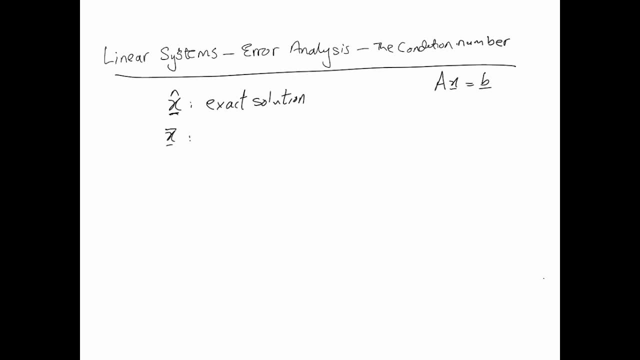 is our approximation, okay, our approximate solution. so we'll call this our approximate solution. and of course, we know that ax is not necessarily equal to b because our solution is approximate. then how can we, in the absence of the exact solution, how can we know how good or how? 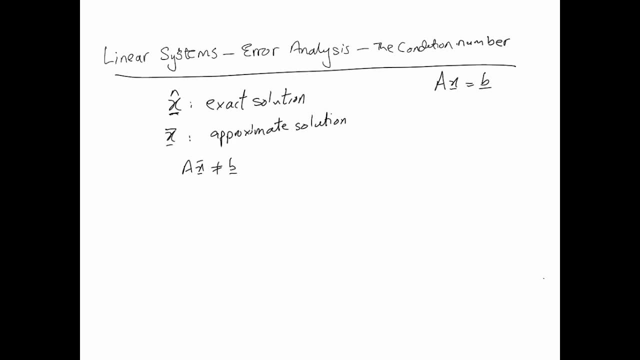 good or bad. our solution actually is for this purpose. we define something called the residual. okay, residual and the residual is basically very simple idea, if you think about it. how can we judge that? we have very simple. we have the right hand side and we have the system ax equals b. now, if i were 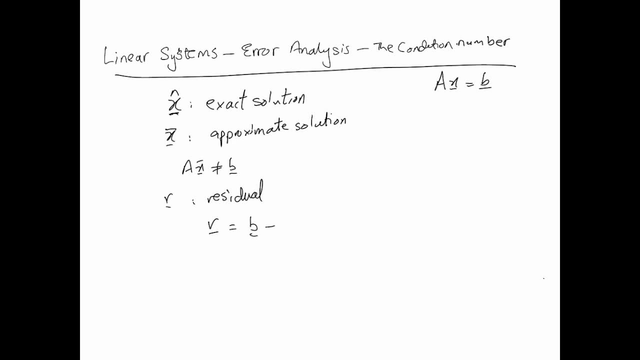 to look at what is the difference between b and ax bar. that should give me a reasonably good idea about how good or bad my solution actually is. now, in order to look at this symbolically: is there actually a relationship between the error in this? let's look. so i'm going to put a box around this. 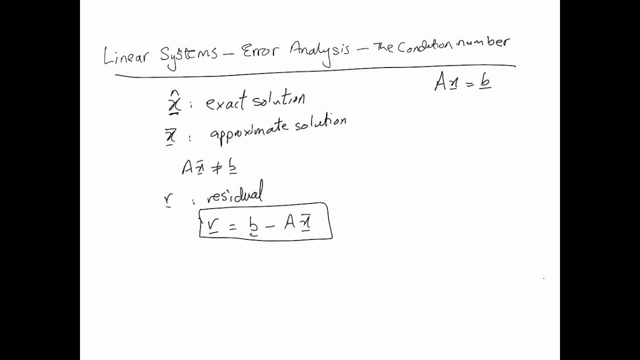 this is the definition of the residual. how we calculate the residual is we take the right hand side and subtract off from it a times our approximate solution. that gives us the residual. now let's have a look at a little bit more detail in this. now, if x- hat is the exact solution, then clearly ax would equal exactly b. it would exactly. 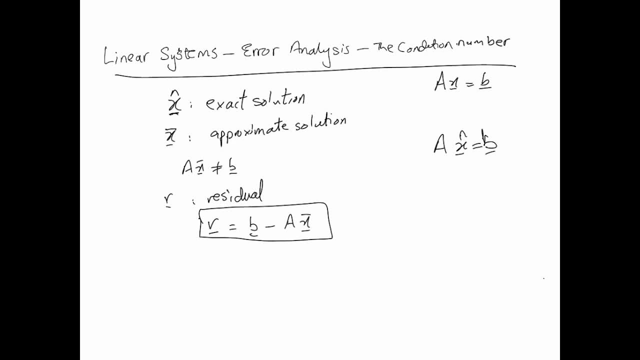 equal b, because this is the exact solution, so it should satisfy the equation perfectly and therefore ax hat should be equal to b, which means that i will be able to calculate the residual. i would be able to just do this, which is: replace here the ax hat and of course then i just have this: 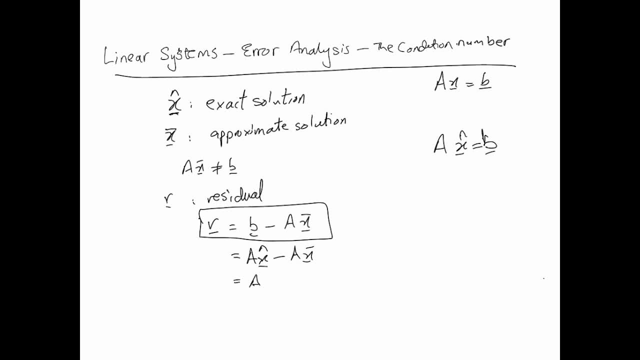 equation revised, which means that this would actually equal. if i take the a out x hat minus x bar our approximation. and now, if i define the vector epsilon as my error, then clearly the error in fact- which you can even see here, by the way- is that if i take the a out x hat minus x bar, 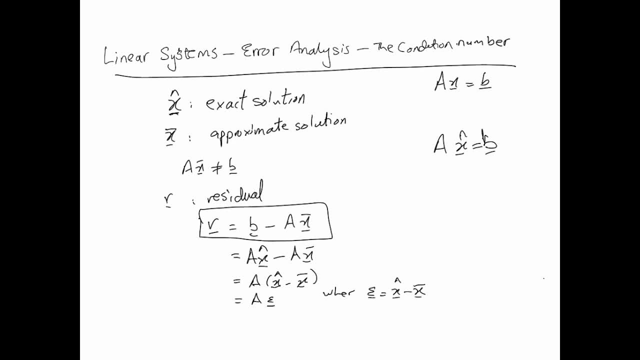 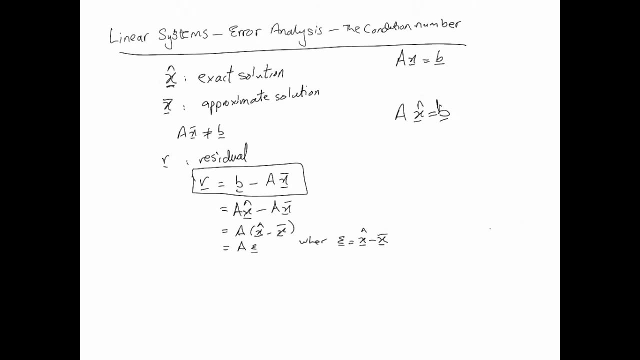 which means that if x a hat equals x bar k one times k is equal to real x hat honor. this is still the original solution. i mean, if that means it is equal to xing, right, so you can say that in the extension, путin did not just with this example, we simply 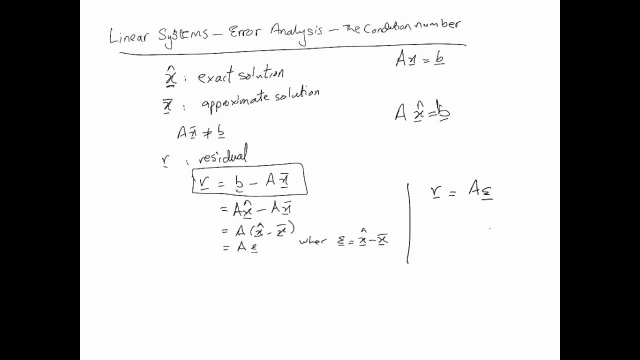 wrote the egalization theorem and in here we are加 x to the union, 한 to the equation and we have again that difference between the exact and the approximation question relationship. this matrix, our coefficient matrix, a times the actual error, and the error is what the error is. 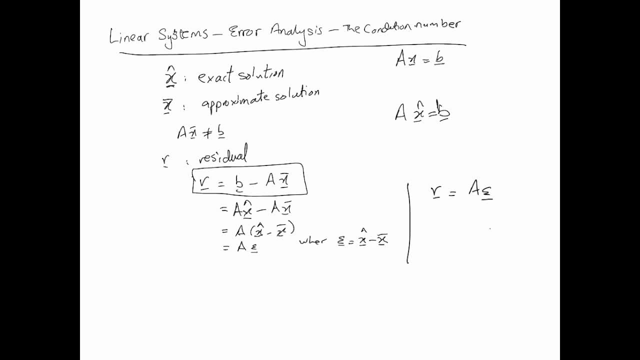 the difference between the approximate solution and the exact solution. now we don't have epsilon because we don't have the exact solution, but we do have and we are able to compute the residual. so the residual, therefore, in theory, should be able to give us a pretty good idea about how good or 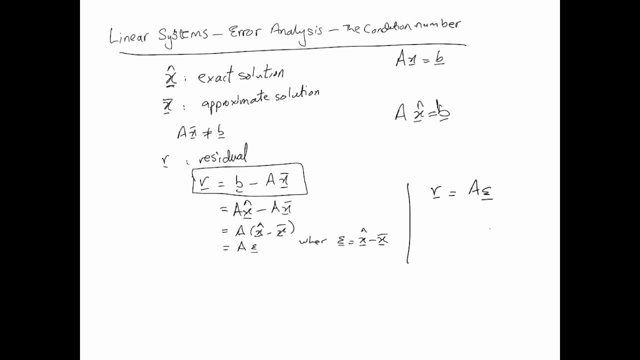 bad. our solution is: well, you think that, but there is a disease that exists within systems of equations and that is called ill-conditioned, l conditioning or ill-conditioned a matrices. so, in other words, this matrix a could be ill-conditioned. so, in theory, epsilon, a small 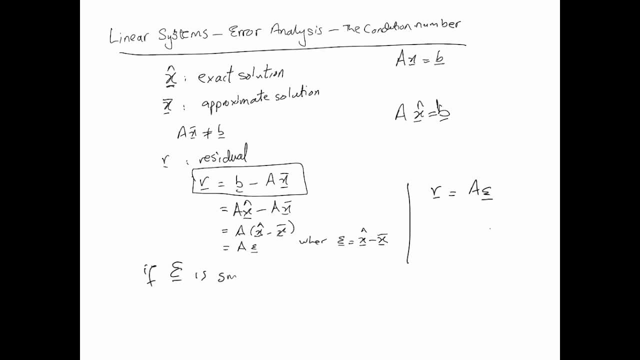 if epsilon is small, okay, that clearly would indicate that r is small, but is the converse true? what can we for sure say that if r is small, what can we say about epsilon? the problem is not always small, and this is a very important problem for us to tackle now, of course. i'll show you by example in: 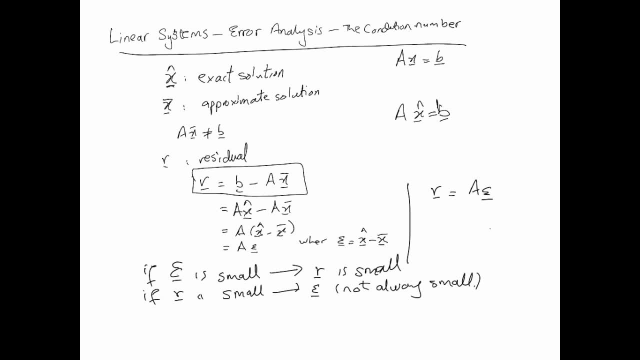 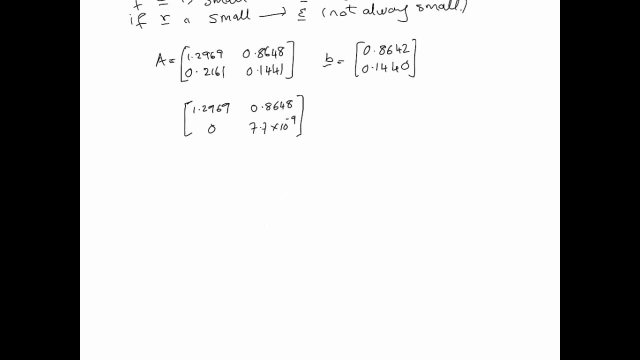 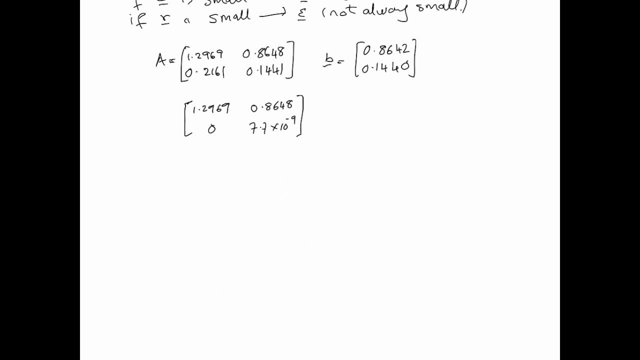 matrix, one iteration of gaussian elimination. one iteration of gaussian elimination would give us this. so as we eliminate, um, as we eliminate this, uh, here we'll make it zero. what happens to the 0.1441 is it becomes 0.7.7 into 10 to the minus 9.. now, that's a very, very small number, in fact. 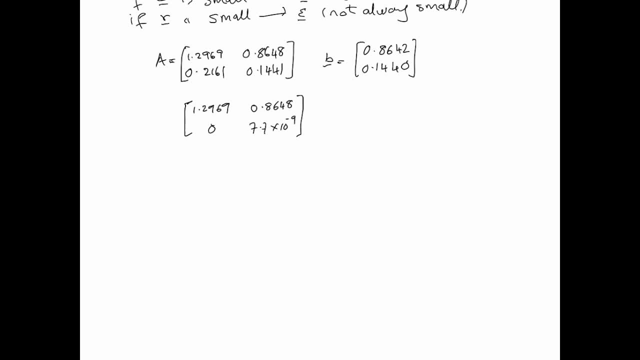 that's almost showing that this matrix a is almost singular, in fact, and a singular matrix means the inverse doesn't exist. so here, if i let me just go further and say that, in this case, when i solve this system, when i go, when i go further and solve the system, okay, 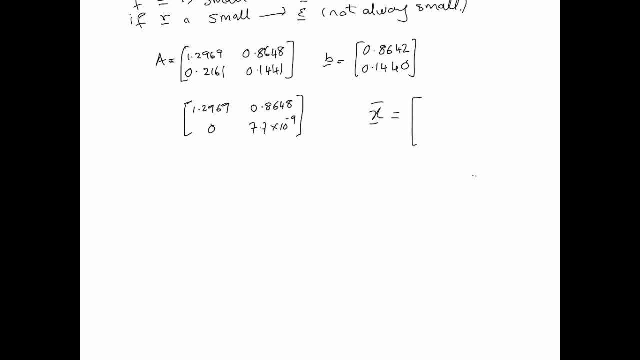 it turns out that the approximate solution- okay, and you can check this yourself- the approximate solution turns out to be this: okay, this is the approximate solution. and now, since i have the approximate solution and i have the a, i can consider it, calculate the residual, which is b minus a times this x, this one here and this a here and this b. 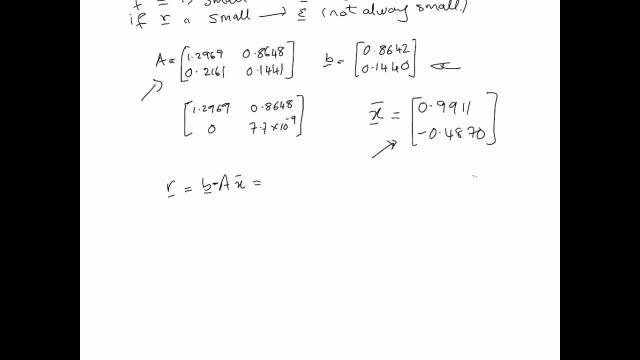 here i take these three, sorry, b minus ax, and when i calculate that turns out that's a. that's equal to 10 to the minus 8, and this is almost 10 to the minus 8. now, that's a very small residual. that's a small residual, okay, that's a small residual. now, if i go further and actually 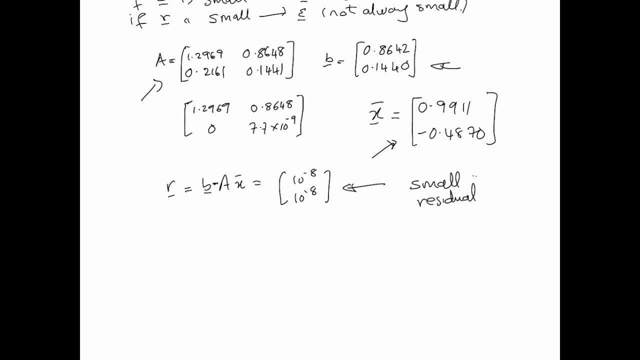 look at the exact solution. the exact solution for this happens to be 2 minus 2. you can check that. look at our solution. our solution is here. this is our approximation and this is the exact solution. the error, okay, in this case, the error in fact is the error in fact is this okay. so, as you see, that's a pretty. 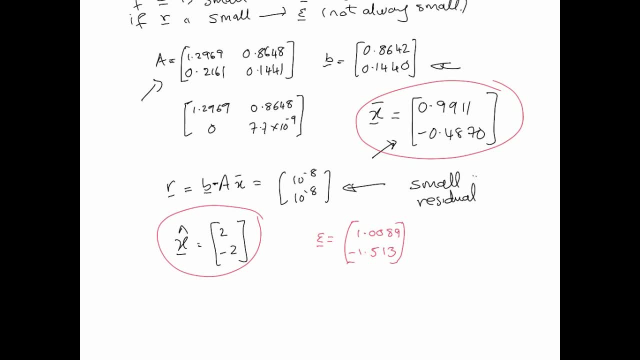 bad error, in fact. so a small residual doesn't necessarily imply a small error. now, what's wrong with this matrix? if we look at this matrix a bit more carefully, if i go back to the point i was trying to make, if you look at this number here, this is the culprit, or in fact, this is the culprit. 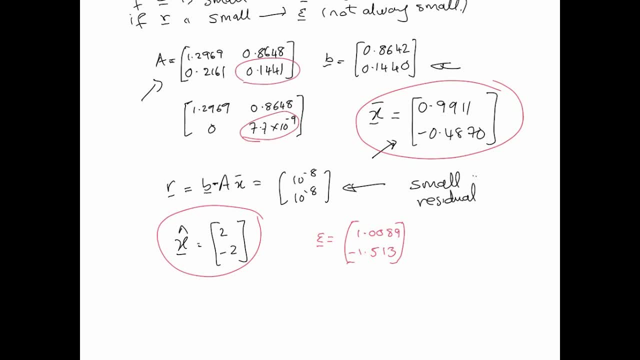 very small changes in this number can lead to very large changes in the solution. in fact, and such a matrix where- which is almost coming down to be where a is almost very nearly singular- we say that a is ill conditioned, ill conditioned. now we need to elaborate on this idea. what is this condition, this ill conditioning that we're 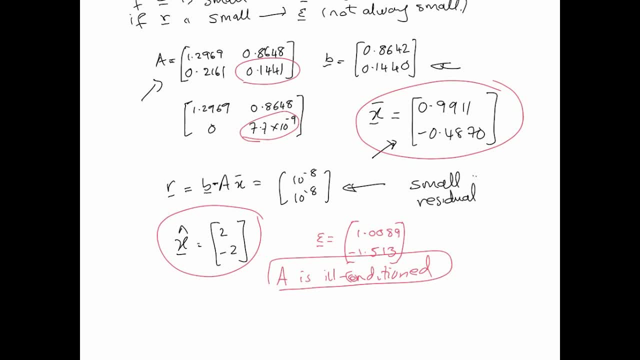 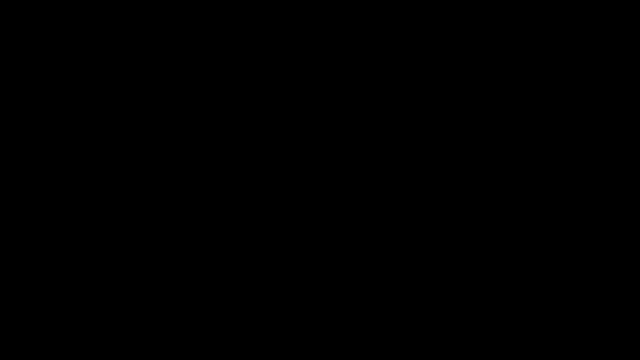 talking about. well, in order to look at this, we need to look at some more preliminaries and then we'll proceed to calculate, in fact, what we initially refer to in the title as the second part of this problem. so here's a question as a continuation of the first question. 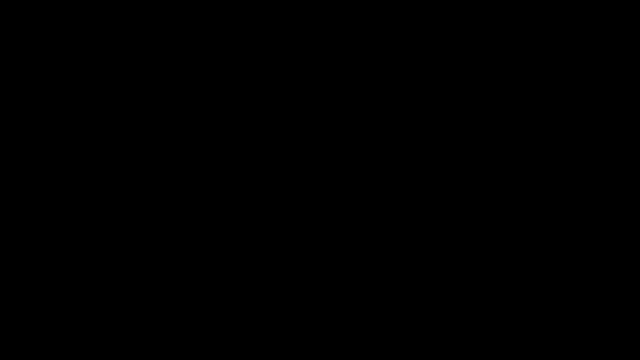 here we'll look at the problem that we initially found. you say the sentence will be taken in the parent search function and then put it in the parent search function and then from there we have this variable, which we call the basic variable, which has this variable, its value, and that's what we're going to do here for this problem.